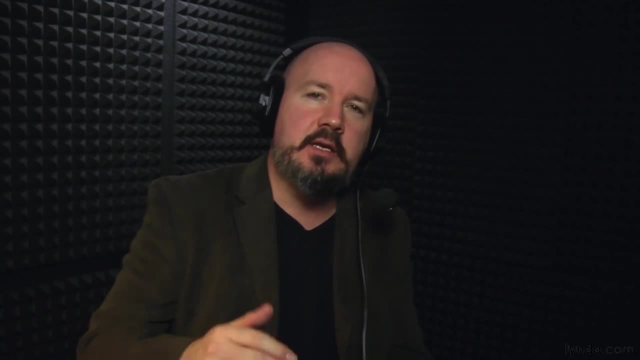 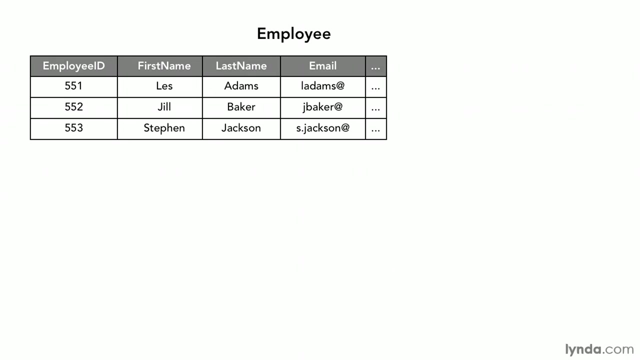 one value, just one value, and there should be no repeating groups. Okay, what does this actually mean? Well, let's say I begin developing a database for my company and one of my tables is an employee table. Very simple stuff: Employee ID, last name, first name and so on. And we 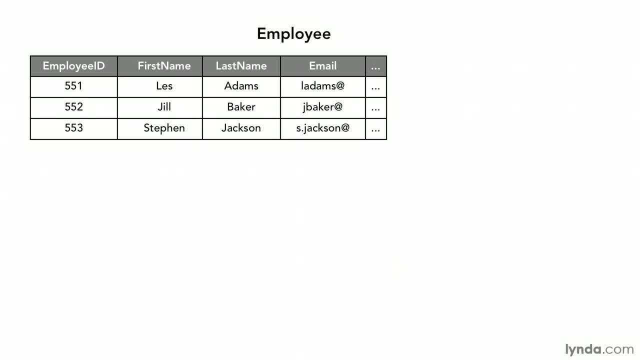 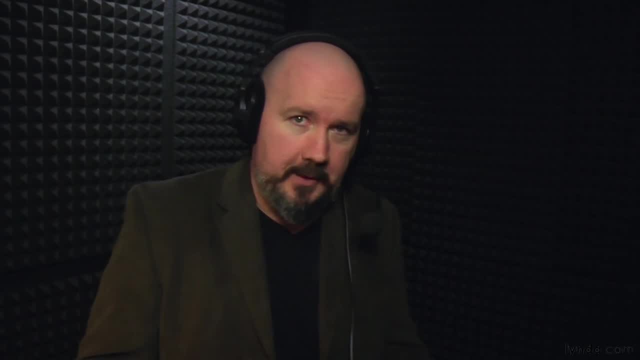 allocate every employee a computer. I want to keep track of that. so we'll add a computer serial column to keep track of who has what. Now this is actually okay right now. This technically is in first normal form. Here's the problem. Let's say, I figure out that some of our employees need 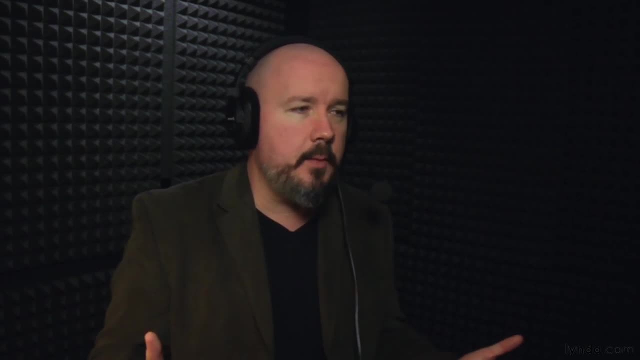 a Mac and a PC to do their testing. Others need a desktop and a laptop. So several people have multiple computers and I want to keep track of all of them. There is a couple of ways that I could deal with this. I could just start stuffing extra data into that one column. We could start. 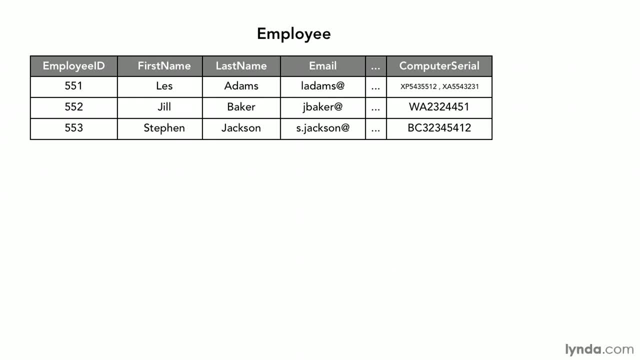 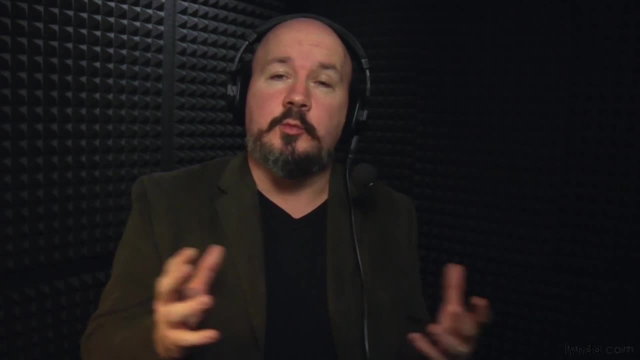 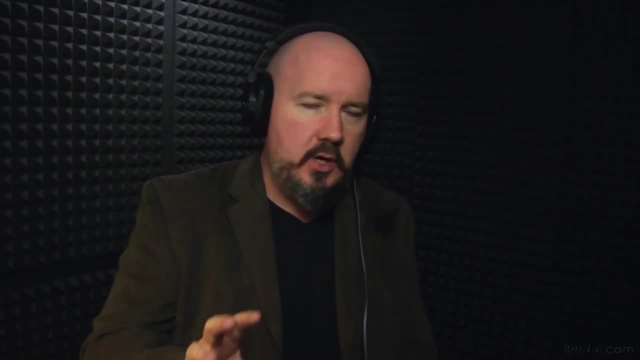 same thing. They'll do the same thing, And they actually deal with hundreds of tables. Each table could have hundreds of columns and millions of rows, but they do not want columns that have a variable amount of values. Perhaps there's one value, Perhaps there's two in it, Perhaps there's. 10. Each column in each row should have one and only one value. Now could you do it this way? Sure, Technically, if that column was defined as character data, the database wouldn't stop you from entering commas and multiple values into it. But as far as the database is concerned, it's still just one value that just happens to have commas in them. So you would find it hard to search directly for a serial number. You'd find it hard to sort, You'd find it hard to maintain. 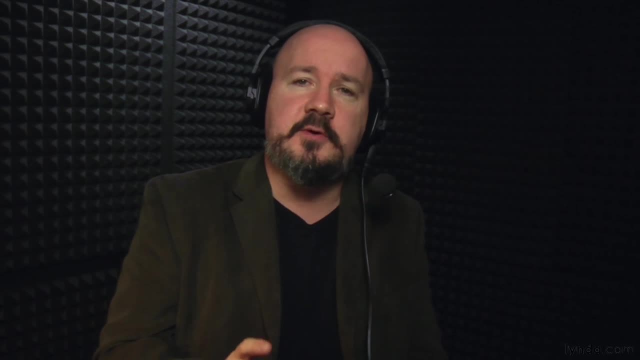 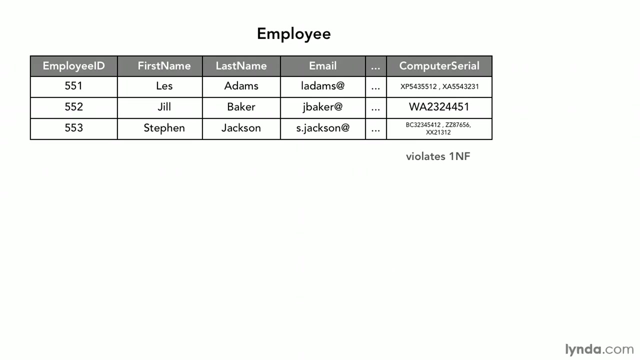 So it's not in first normal form if you do this, because first normal form demands that every column, every field, contains one and only one value. So what we might do then is go back to the original way and instead start adding new columns. 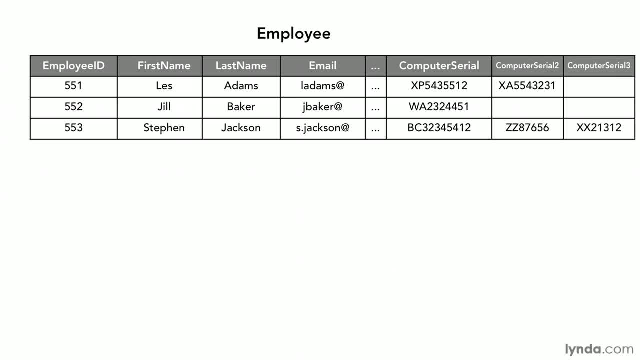 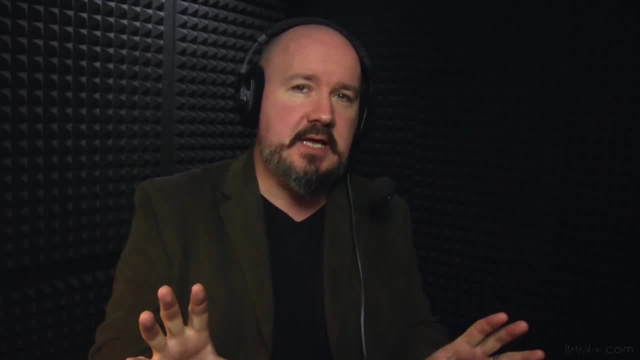 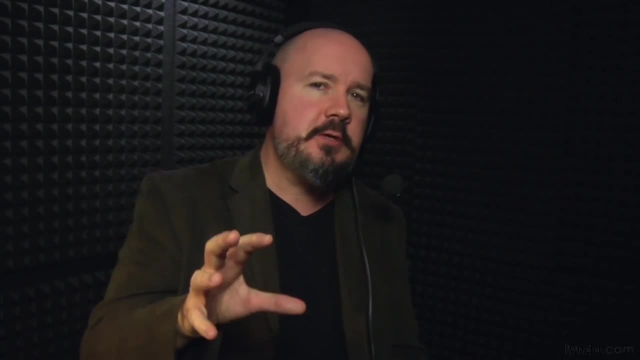 So computer serial two, computer serial three. This is what's called a repeating group and there should be no repeating groups. The classic sign of a repeating group column is a column with the same name and the number tacked onto the end of it just to make it unique, because usually this is a sign of. an inflexible design. Sure, if we could guarantee that there would only ever be two or three, that's fine. But what happens when we want to add the tablet and the smartphone? What happens? What happens when one employee manages testing and needs to be associated with six computers?